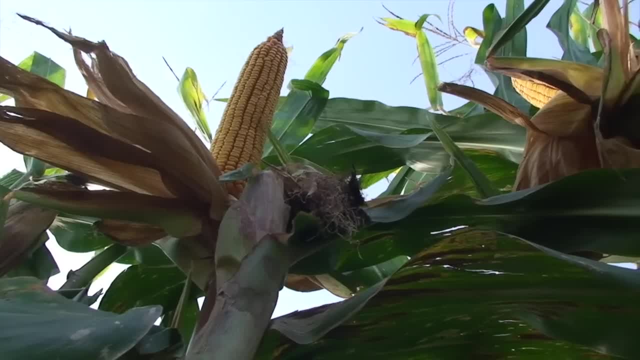 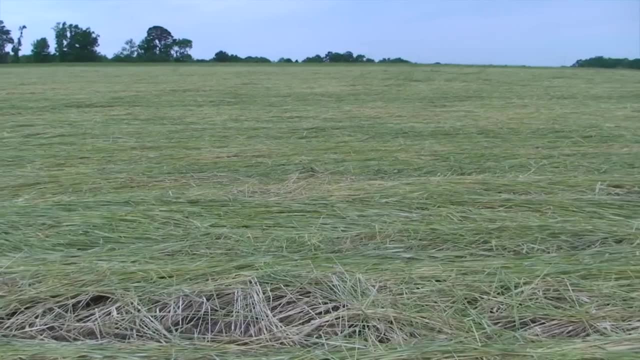 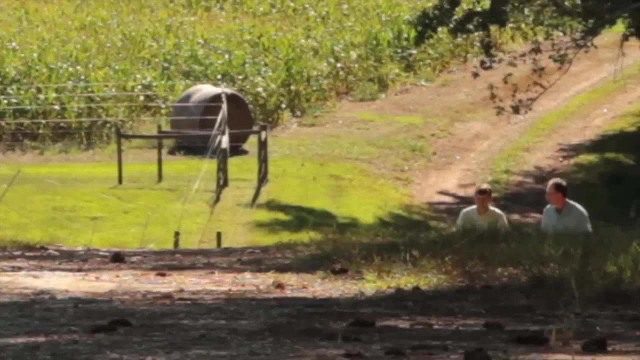 No cropping system is drought proof, but there are things that farmers can do to mitigate the effects of a dry year. The road took us to NC State's Dr Chris Rehberg-Horton to discuss how cover crops affect water dynamics. Water, I think, is going to be real limiting factors over the next. 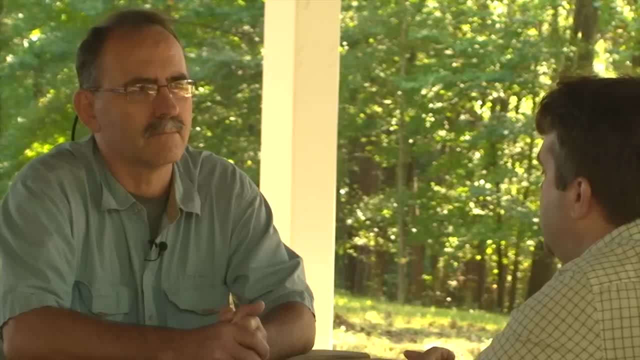 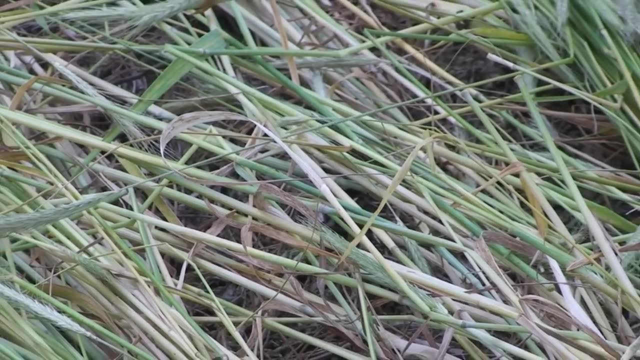 several decades, and particularly here in the southeast, we tend to get most of our summer precipitation and these huge rain events, and one of the things that cover crops bring to this system is they slow the movement of water across our fields and so that we think that we have a 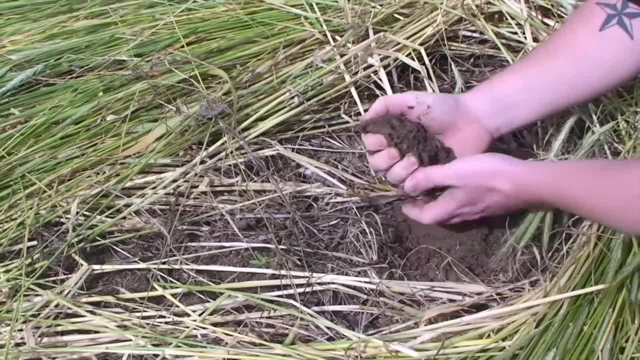 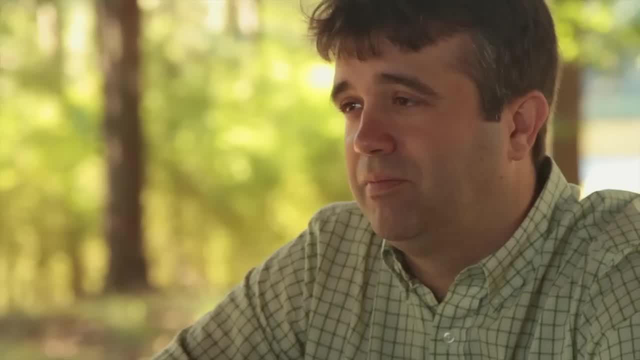 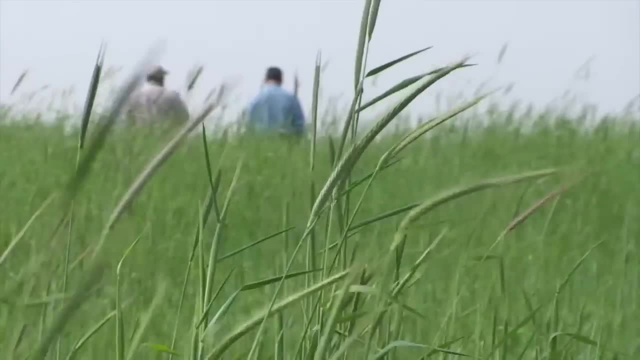 lot of yield potential that we can garner with cover crop residues, by allowing more water to soak into the soil. Okay, okay, Well, tell us about some of the actual work that you've done. Sure well, we've worked both in corn and soybeans at this point, So we started with soybeans. 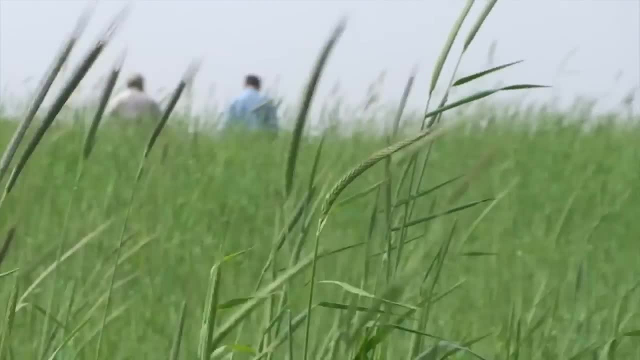 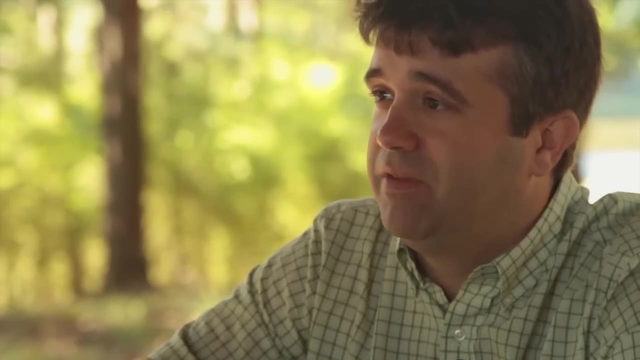 and there we use a rye cover crop. One of the ways that we're going to get more biomass into these systems is not treating the cover crop as an afterthought, Thinking of it as a key part of the production philosophy of the field. We plant our rye cover crops early, which makes a big 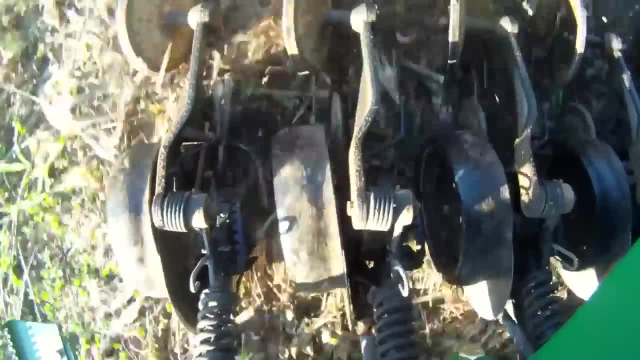 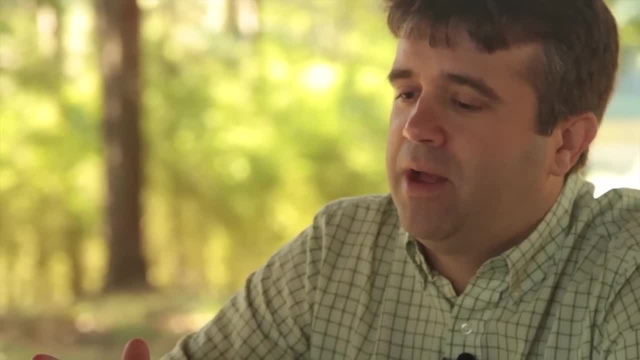 difference. We try to plant that in October as opposed to throwing it in. you know, November, December time frame. That does tremendous amounts for us. It's interesting what that does for water dynamics, I think. for one thing, it makes it actually drier in the spring. If you think about 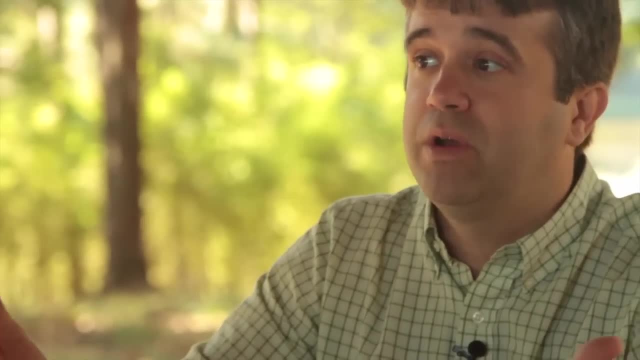 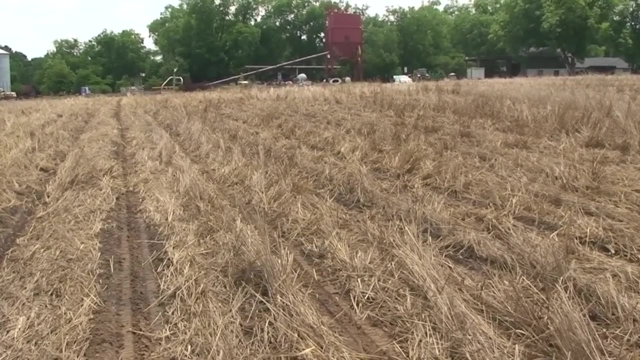 it. if we plant a plant out there over the winter and we're going to grow it, we're going to, we're going to extract water out of the soil over the season. So as you plant, we can actually be a fair bit drier than we would be Now. that can be a plus or minus depending on where you're farming. So in 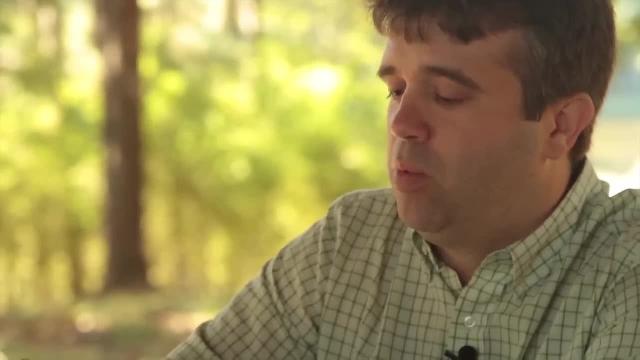 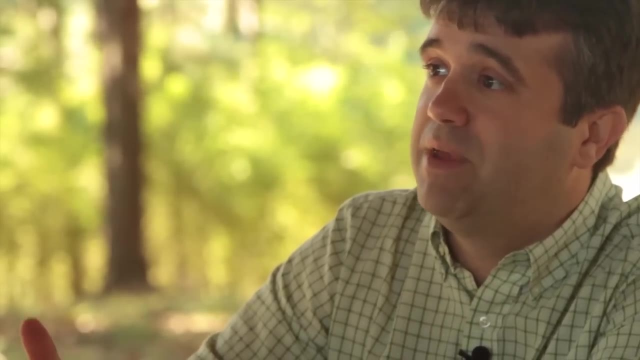 some areas you know traditional no-till agriculture. without the cover crop we can be a bit wet and cool later into the spring And so getting into the field can be a trouble. So some drying can be a benefit on some soil types. On some soil types it can be a greater concern.